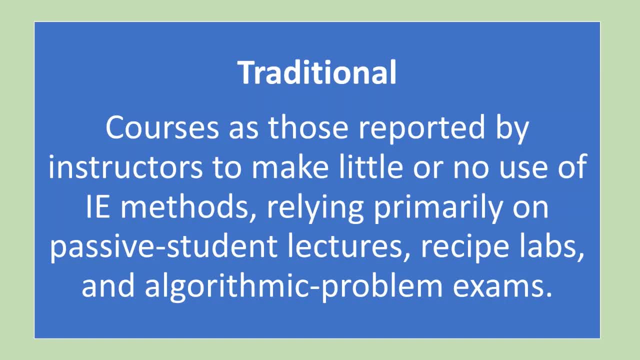 recipe labs. follow the instructions. algorithmic problem exams. I don't want to get too provocative, but of course some people might recognise the concept. but I don't want to get too provocative, So I'd like to recognise some of the approaches that are being suggested in that traditional as 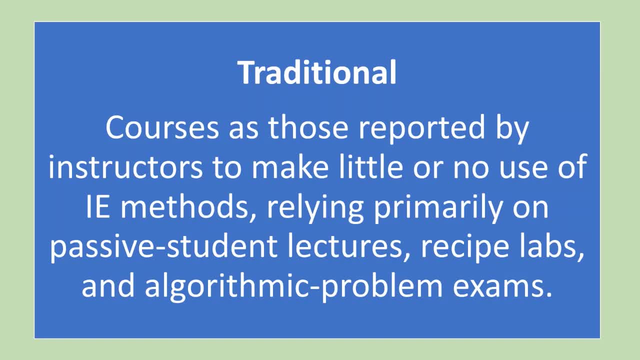 aligning with what might be referred to as direct instruction. I would take a little bit of issue with that because I think direct instruction is perhaps being misrepresented. but broadly speaking, the teacher takes control, teacher reads stuff out. So we compare interactive engagement to. 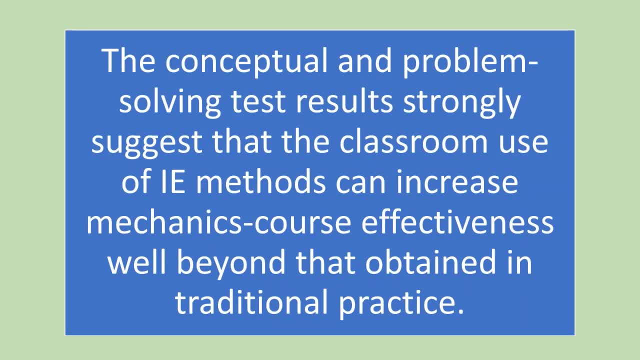 traditional. you compare them and it turns out that interactive engagement is better. Now, better is a problematic word. If anyone has spent any time looking at any set of data, we'll know these are sample populations. There'll be a great deal of overlap, but broadly speaking, 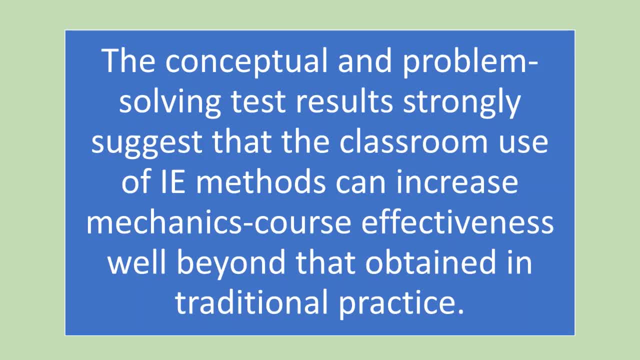 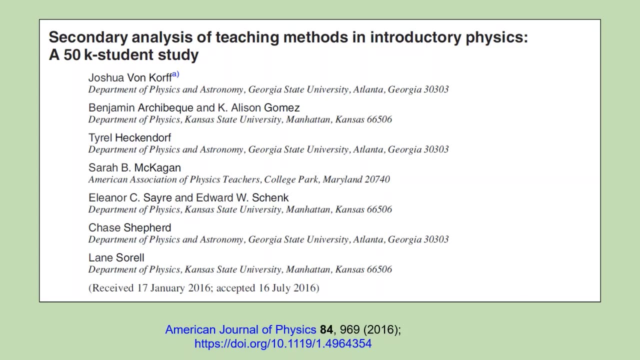 it seems the interactive engagement approaches, as outlined earlier, yielded better learning gains than the traditional approach. And if that sample size wasn't big enough for you, this work was revisited in 2016, and they looked across a wider range of contexts. So, in addition to sort of the comparison between interactive engagement and traditional learning. they looked across a wider range of contexts. So, in addition to sort of the comparison between interactive engagement and traditional learning, they looked across a wider range of contexts. So, in addition to sort of the comparison between interactive engagement and traditional, 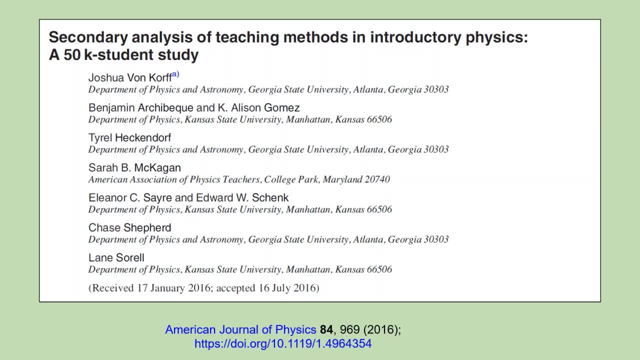 lecturing. this version of the study also looked at different contexts and different environments to see whether that made a difference, And it turns out, broadly speaking, no Turns out. the interactive engagement appears to be a more efficacious way to teach mechanics. introductory. 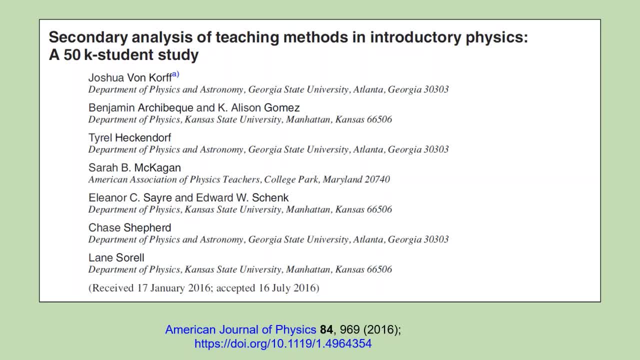 physics than the lecture-style approach. Now I'm always cautious in saying, oh, you must teach this way. but what I would say comes out of this paper is we do have a large scale study, rigorously done, reviewed in multiple contexts. that suggests a particular 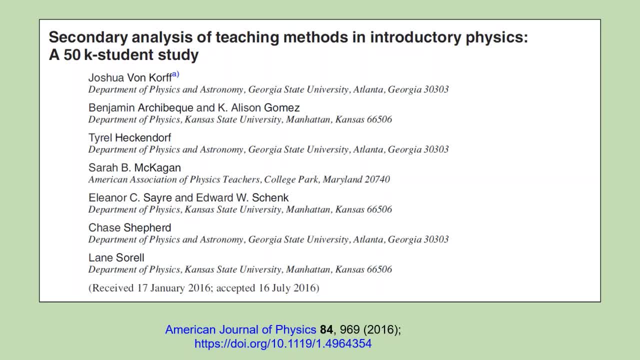 approach to teaching mechanics is more likely to help students learn than another one. Interactive engagement appears to be a better approach to teaching that particular topic than the more traditional lecture style do: lots of questions and more questions, and more questions. So I don't offer that as a you must do it. I offer that as a provocation to reflect. 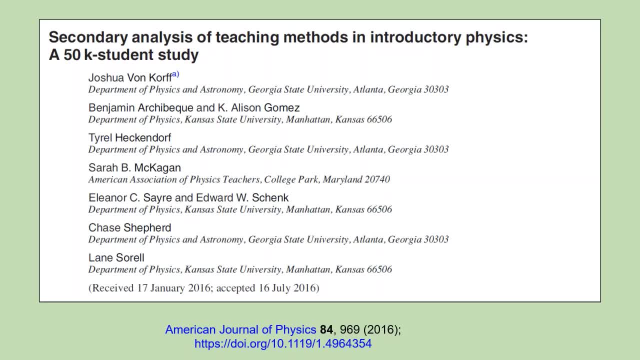 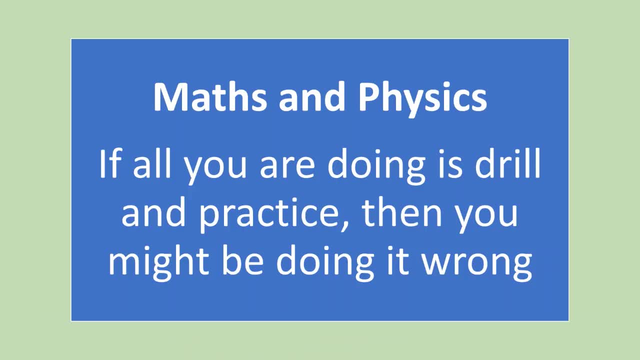 and when you're thinking about planning your topic here, maybe you should be starting thinking about what's in the original study, in here referred to as interactive engagement, And following on from that, I'm going to take the line about doing lots of questions a little bit further and talk about the role of maths. 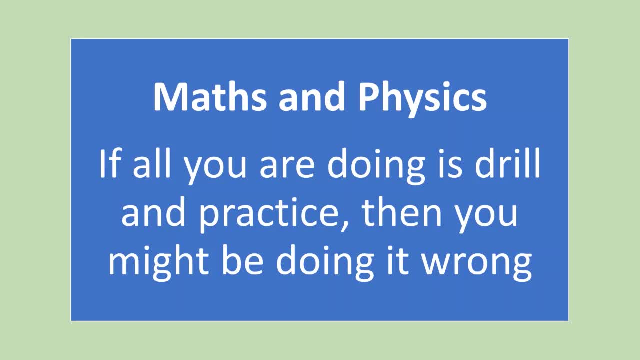 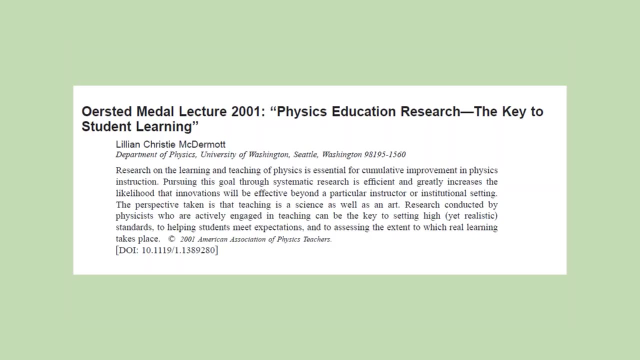 in physics and suggest that if your view of the mathematical side of physics is to get students to do question after question after question, I'm going to suggest there's a potential problem there And I'm going to draw my argument from two places. The first is from a lecture from 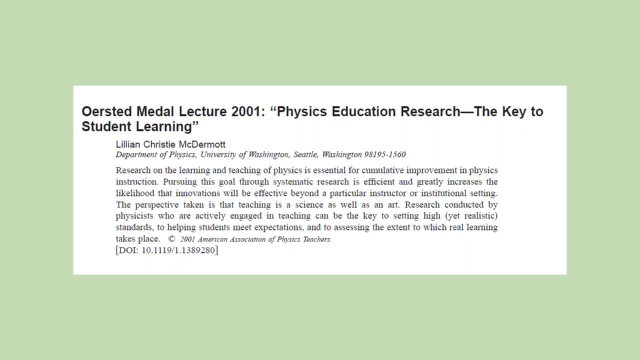 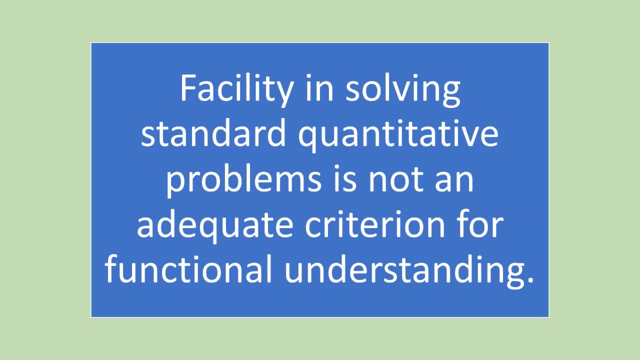 Lilian Mcdermott in 2001.. Lilian was one of the kind of giant brains in physics education research. She's quite blunt. in her view, being able to do standard quantity problems is not adequate. It doesn't mean it's not needed. Of course it's needed, but it's not enough. 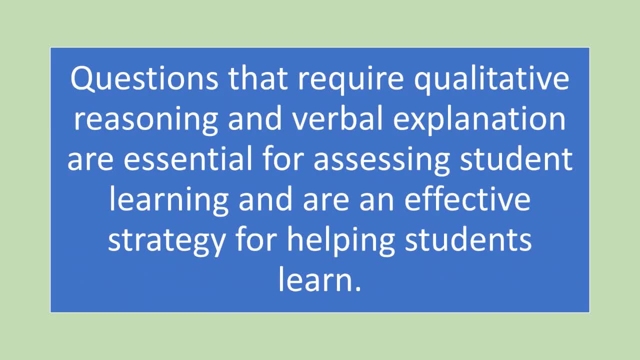 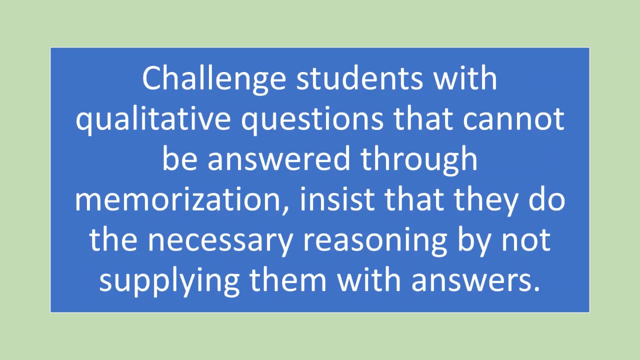 You've got to get students to think about that. You've got to get them to think about these, about their thinking, their reasoning and their answers, both to help them as learners and, in a good way, for us as teachers. give them questions they can't memorize and as a whole slew related to the first research paper. i. 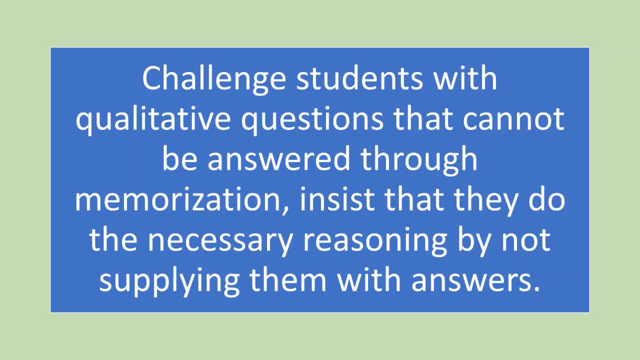 mentioned, but also more broadly in physics. that says that students can do a bunch of numerical questions. you give them a conceptual question, they get it wrong. so this is not just someone's opinion. this is based on evidence. the second person i want to draw into this argument to: 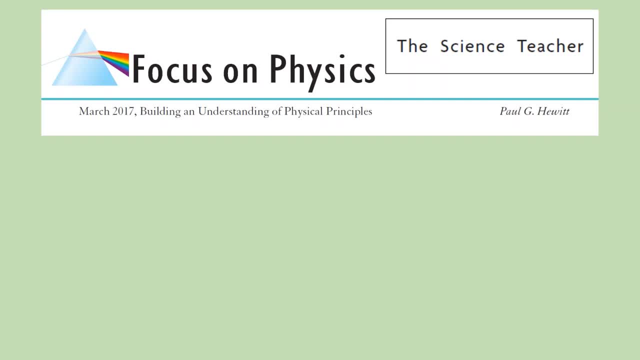 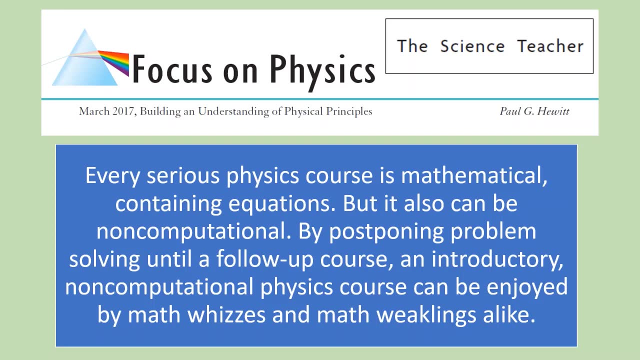 support. what i'm going to say is a person called paul hewitt. now is not the time to talk about how great he is, but he makes a really significant distinction, at least in my mind, between mathematical and computational. the math is there. the math is important. we can't ignore it, that's. 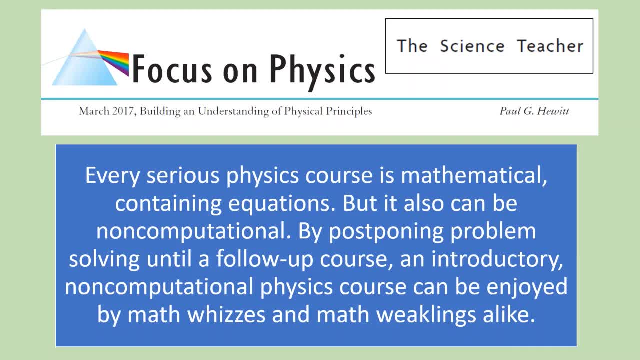 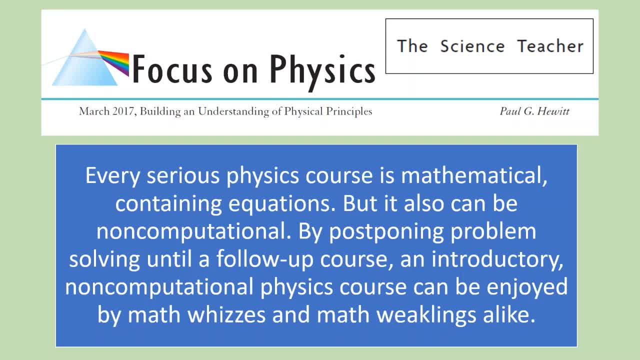 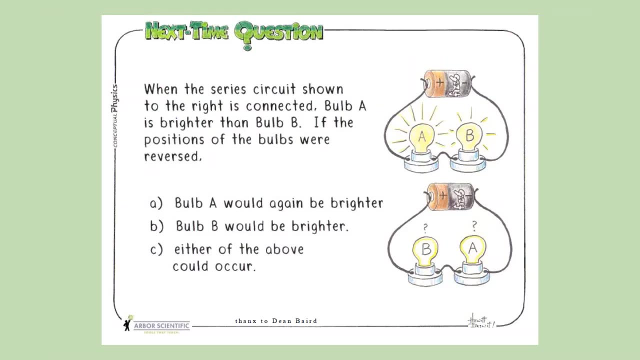 isn't that an impoverished experience of physics? the questions, the numerical questions got to be there, but if you lead with those questions, and that's what students see as the identity, that just seems a terrible representation of a beautiful subject. there's so much more than that, and paul hewitt developed a whole. 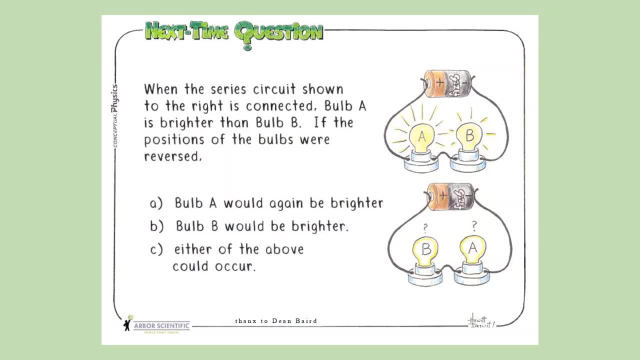 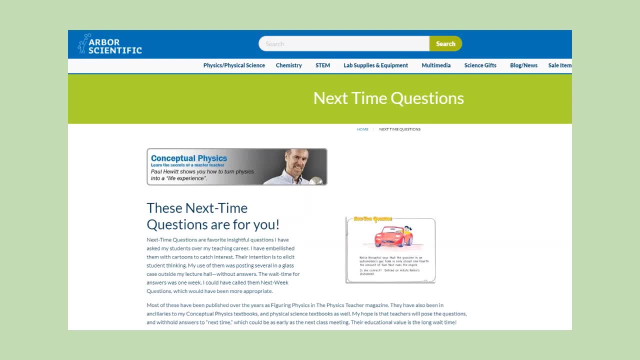 load of questions that are conceptual, that are the kind of thing lilly mcdermott was talking about, that do require students to think they're available for free from the arbor scientific website and they are fantastic- possibly the second most useful website for any physics teacher. 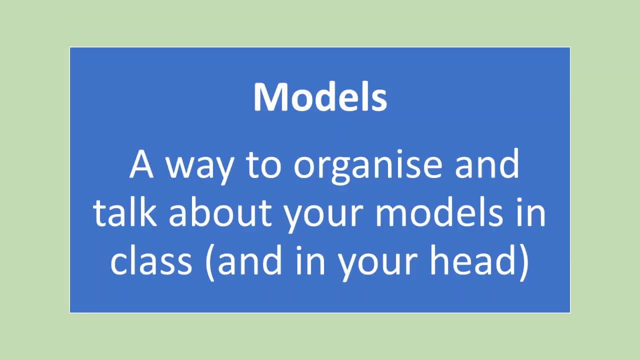 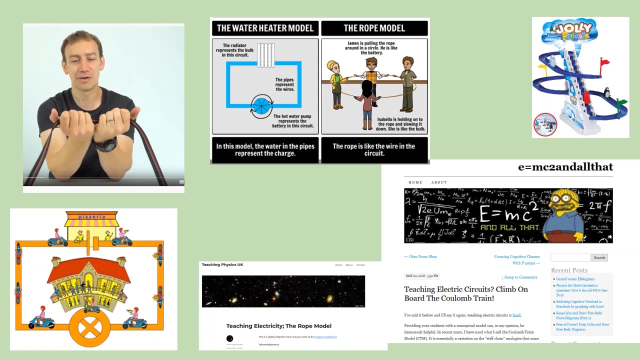 after fett models. i think we're all reasonably confident that the use of models is a very key part of a physics teacher's life. if you're teaching electricity, you could probably, you know, fill a room full of different models and everyone has their own view and i'm not going 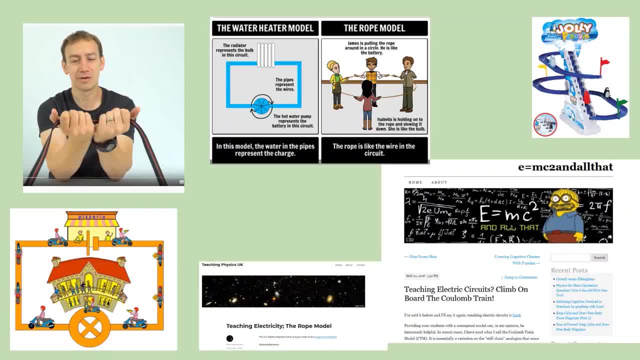 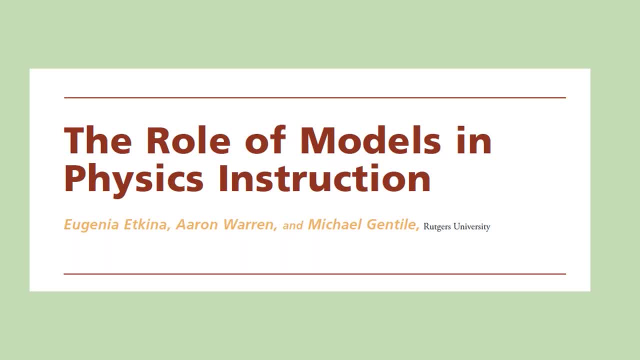 to talk about which is the best model for the moment. i'm going to talk about some ideas that i've borrowed and tweaked slightly from this paper. all three well-respected writers in physics education, eugenia akina. i would make another particular kind of flag wave for us being a 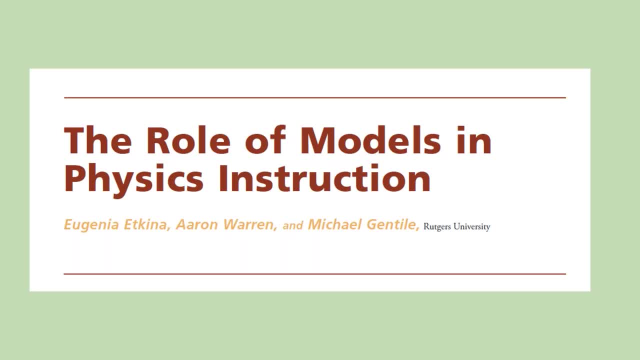 really great brain and mind in physics education. so if you see her name, definitely read anything about her and if you're interested in reading her work, you can read her work and you can find out what she's written and what she's done, because it's it's worth your time. but in this 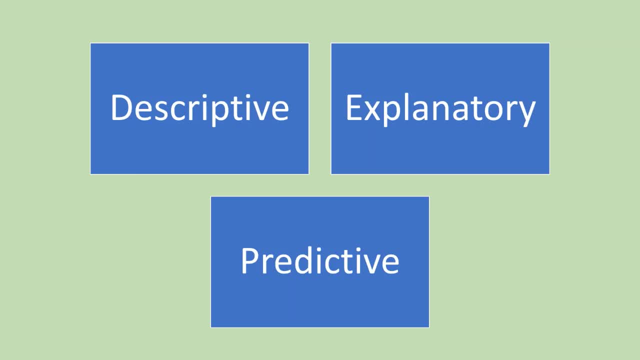 paper. one of the suggestions they make is that you can consider a kind of taxonomy of models, and this is- this is a subset of what they offer, but i think this is the school version. models could be descriptive, they could be explanatory, they could be predictive. some models might be one or more of. 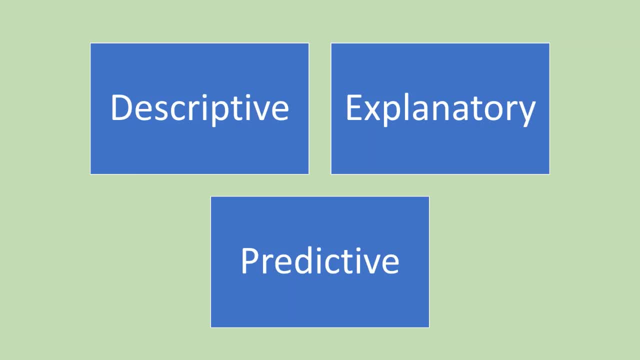 those. some models may have aspects of some of them. so if you take the rope model, for example, i think it's a relationship between the pull and the current and the moving of the rope. i don't think it's explanatory. it doesn't really explain why the electrons are moving and it's kind of quasi. 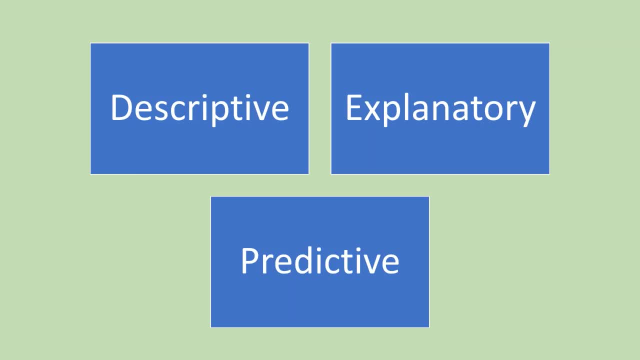 predictive. but the thing i would take from the paper and the thing i would suggest- if i, you know, push this taxonomy on you- is: it's a really good, simple language to think about yourself and when talking to students, it's a way of framing, considering, evaluating and talking about the 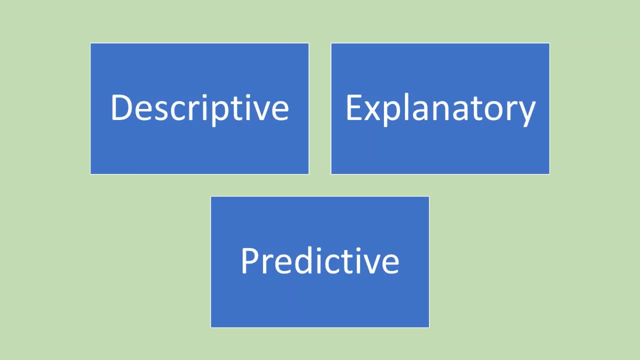 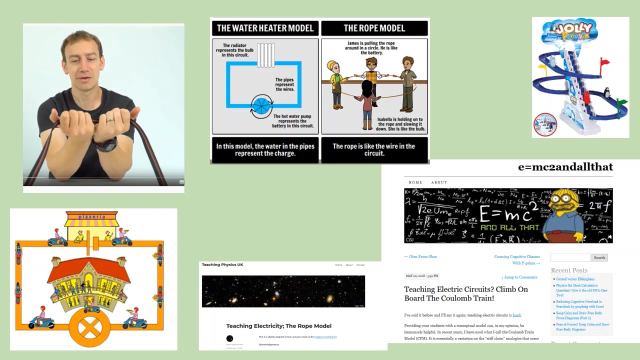 models you use. so you go beyond. this is a model that you know. you think about modeling as a process itself, which is a powerful and important part of being a physics teacher. so when you come back to deciding your models in electricity or elsewhere, i'm going to suggest that three-part descriptive explanatory. 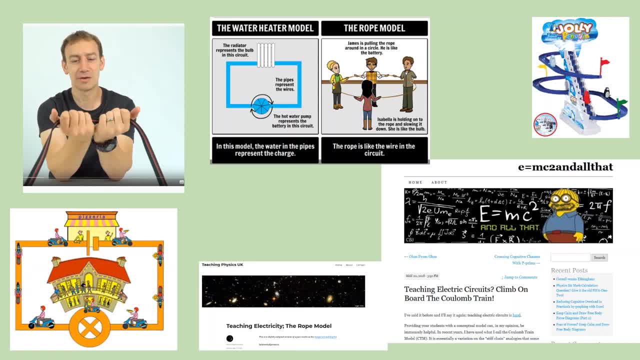 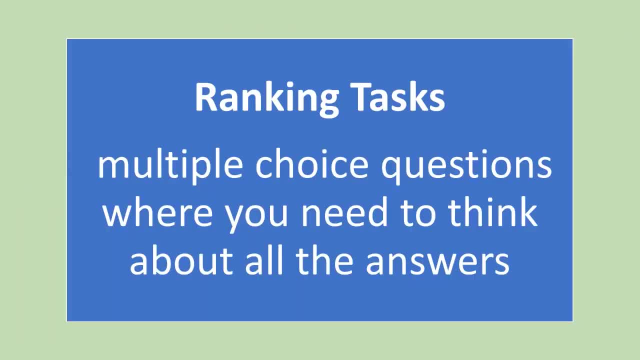 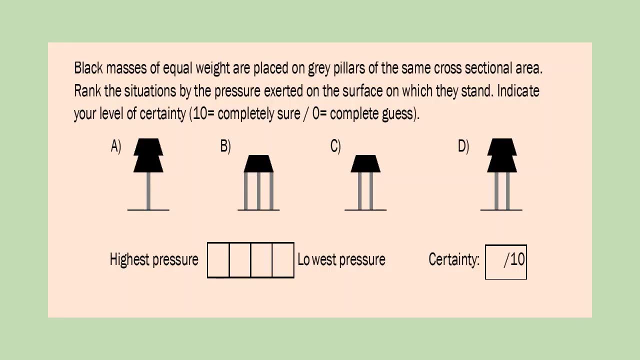 predictive. use that as a way to interrogate your choices and as a way to talk to students about what you think might be a good or bad idea and why. i want to talk about ranking tasks very briefly. ranking tasks are multiple choice questions where students have to take. 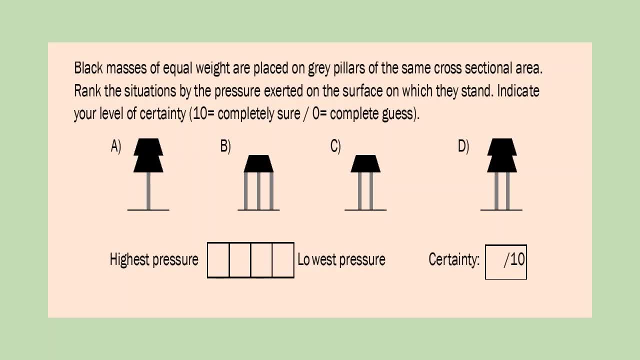 all the answers and order them from highest to lowest or some other kind of comparative measure. what's good about them is they require students to engage with all of the answers, so in a way, all the answers are right. it's just how right they are. so, rather than immediately, 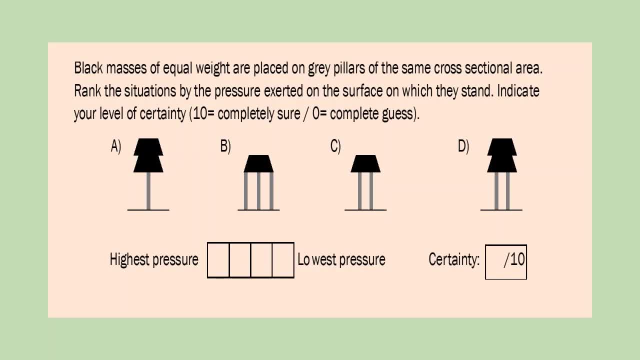 picking a right answer, discarding the others. this type of question requires students to really think about what is going on. this particular one is written by a colleague of mine called richard brock. there are ones available and i'll show you a few in a second, but i think they're really 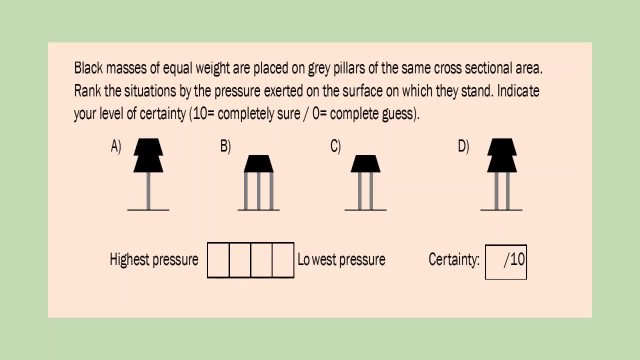 powerful questions because they really force students to think. in this particular case there's a certainty level as well. and just to throw in a kind of teaser to other things that we may get to talk about another day- looking at how confident students are and the accuracy of their response- 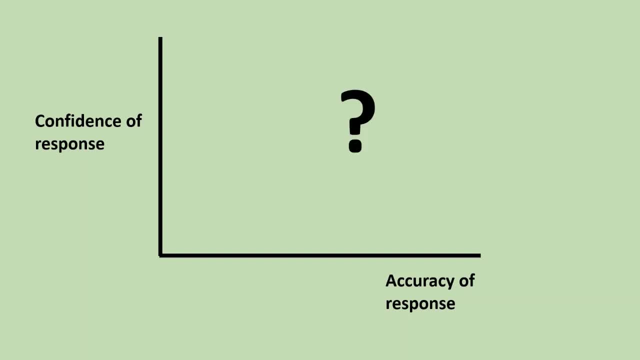 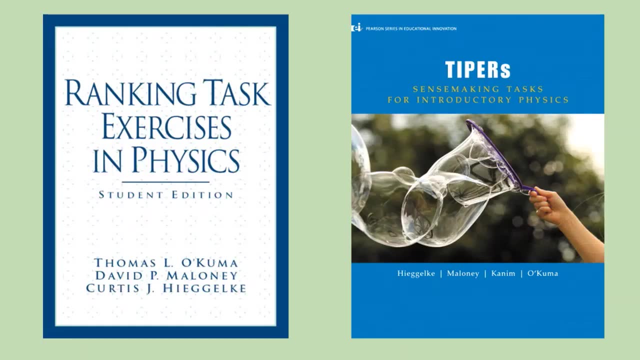 can yield some interesting answers, particularly with respect to individual questions. so i'm going to go back to individual groups. gender is one, but there are other ones. so that question i showed you is written by richard. they do take a while to write, so if only you could buy a book of them. 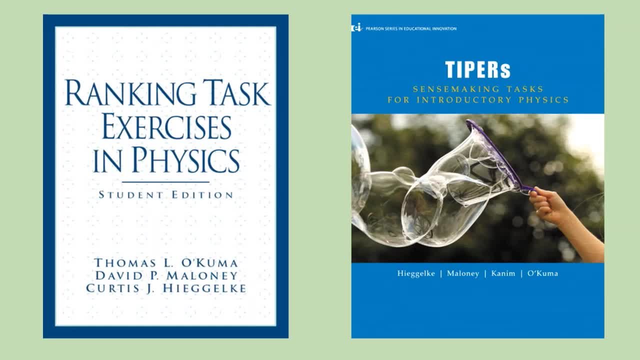 well you can. so there we go. so tippers has loads of ranking tasks and loads of other questions as well. it's a bit frustrating. doesn't have any answers, but that's one that's in print now, whereas the ranking task exercises in physics book. you have to get second hand, but highly recommended. 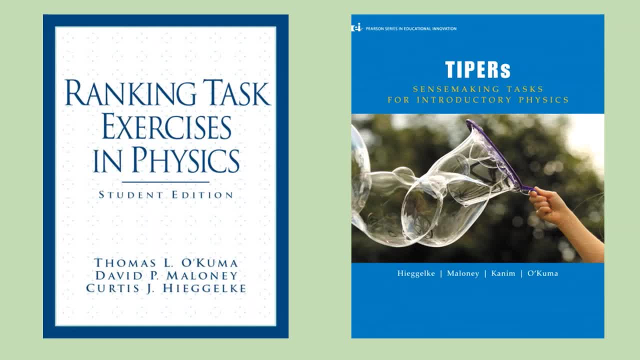 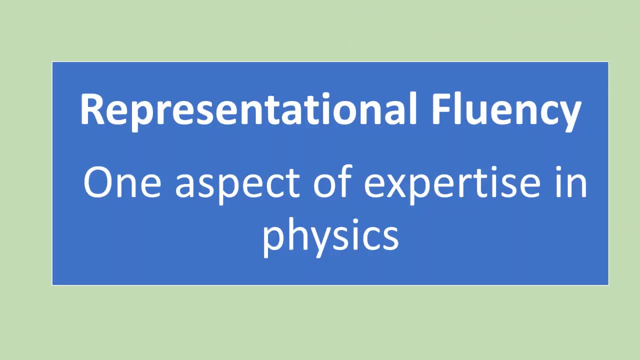 and an enormously powerful and useful resource as well. so i'm going to go back to the ranking task, which i would suggest is a really, you know, well thought through type of question in physics. final thing i want to talk about is what i'm going to call representational fluency, and it's 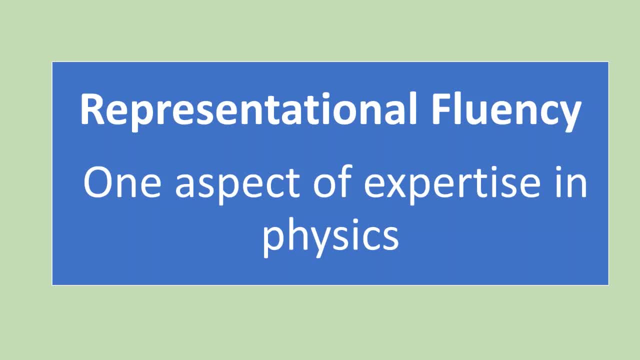 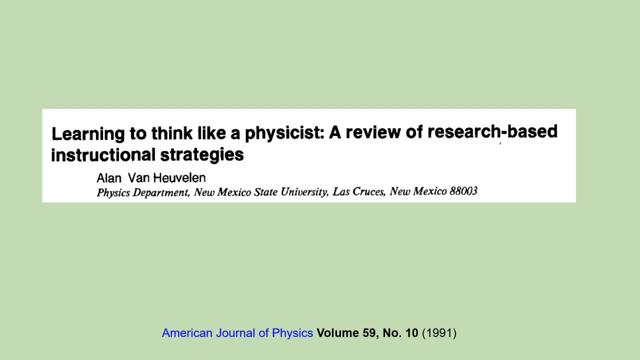 an aspect of expertise in physics or, i guess, in learning physics and teaching physics, comes or is adapted. my thinking is adapted from this particular paper from the early 90s- another well-regarded name in physics education- who tried to kind of cope with or categorize what it was that made people think like physicists in 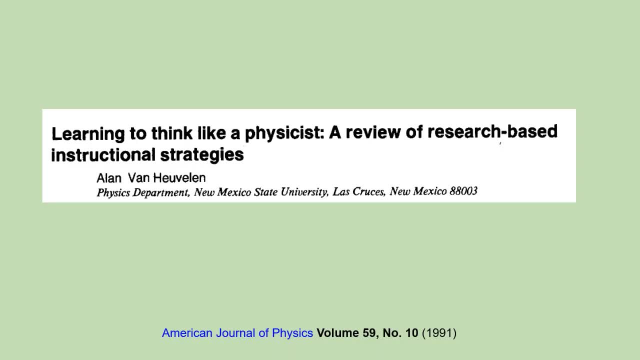 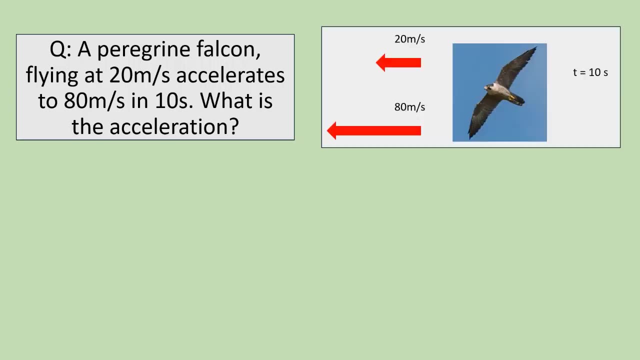 terms of answering questions, but i'm going to draw one thread out. this step paper is definitely worth getting holding of looking at, but it is particularly focused on undergraduate teaching, so it gets quite heavy in places. let's have a question. there we go. looks reasonably familiar that might also having been presented in words. in that first example presented some kind of pictorial. 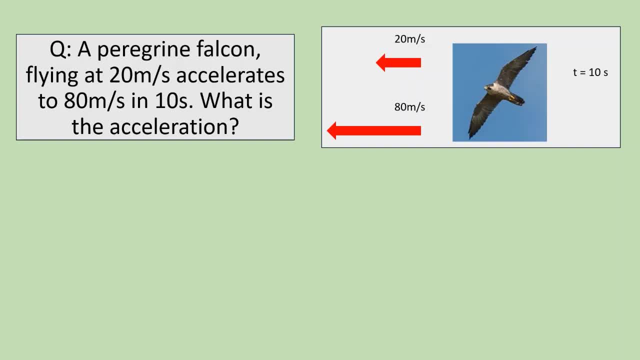 there, but most of you will go: oh yeah, okay, i can see it's the same question might represent it as a graph or it might be represented in a format like that. if you are an expert in physics, you see one question that's represented in four different ways. you can navigate between them. 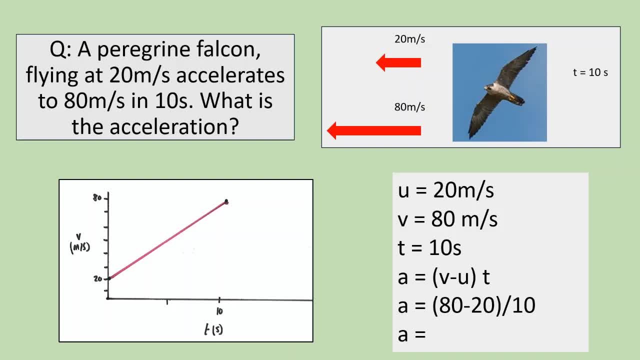 but the deep question, the question that takes me through those is the same to your mind, and the suggestion is from the van heuvelen paper and certainly from other work about expertise beyond physics. if novices see surface features, experts see deep features underneath it. so in this question, someone who is not fluent in physics may well be seeing four different. 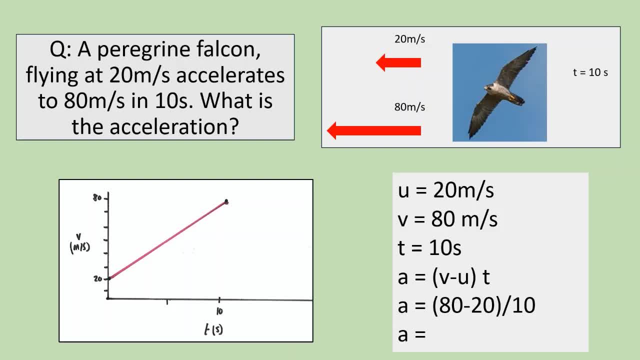 questions. they may not realize that it's the same question even if those multiple representations are put on the same board at the same time. they may not realize: oh, it's all the same thing. that graph is of the perican falcon. those arrows are representing that, those uvts and a's are. 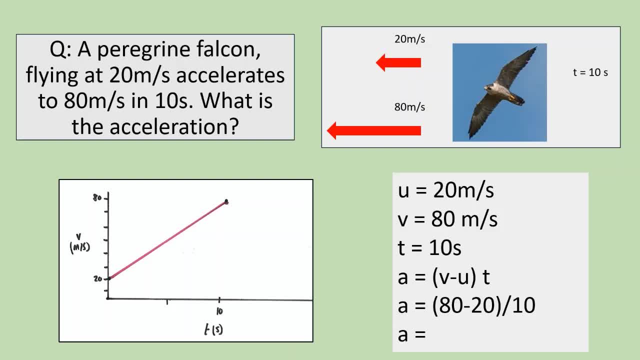 the same question. so one of the characteristics of expertise in physics is the ability to navigate between multiple representations in physics, and so us, as experts, need to think about how we support students in doing that, in realizing that these are multiple versions of the same questions and the same question can be represented in different ways. so that idea of